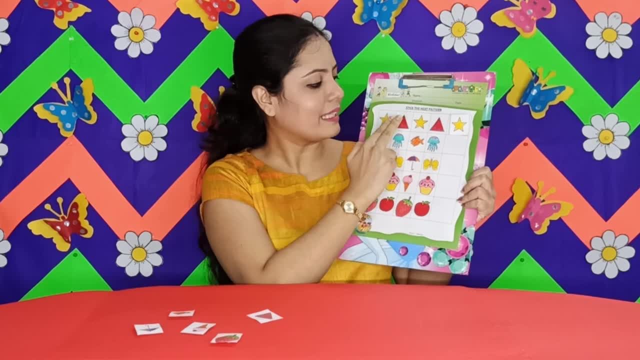 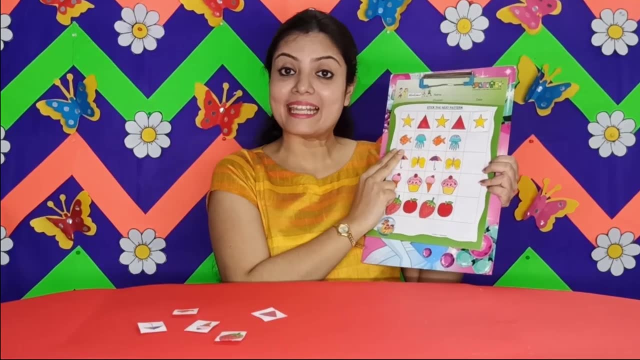 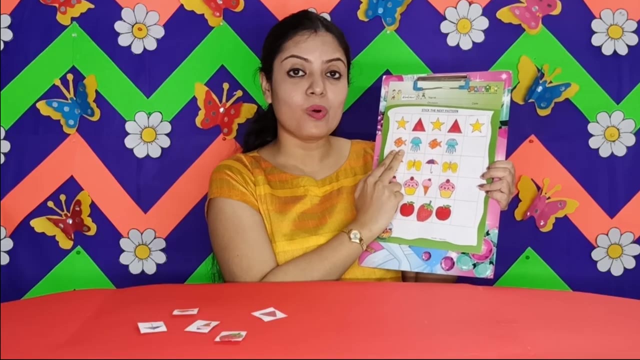 Yes, because there is a star, then a triangle, star triangle, then again a star. So, coming to the next, Look, children, what can you see? This is a fish, isn't it? So what comes after fish? It's a jellyfish. 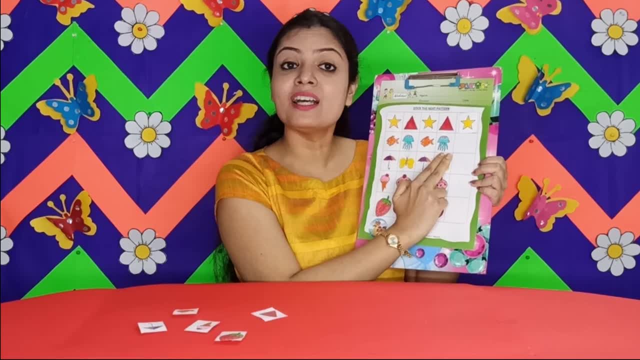 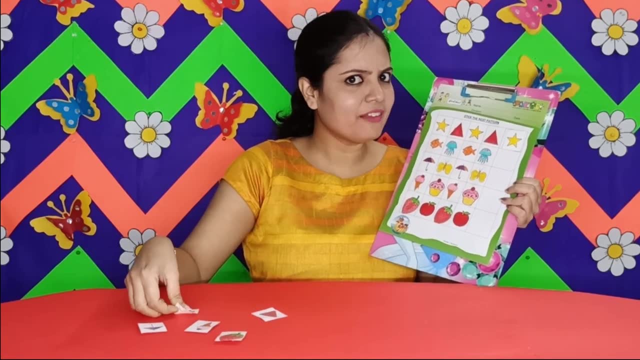 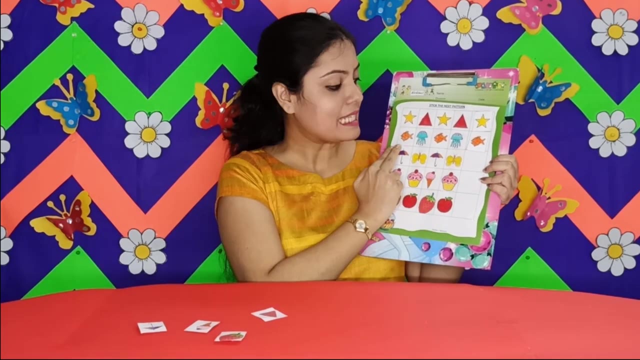 So again a fish, then followed by a jellyfish. So tell me, what will I place over here? Think, think, think. Is it a jellyfish or a fish? Yes, there will be a fish after the jellyfish. See the pattern. 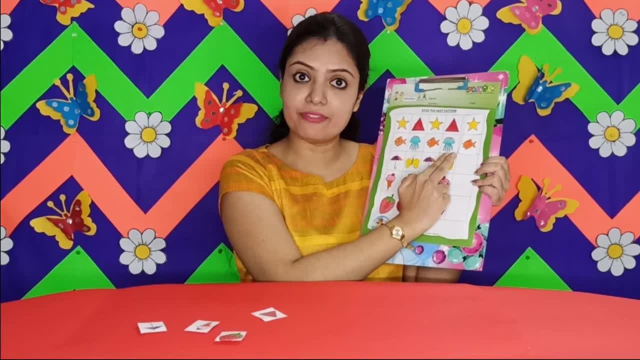 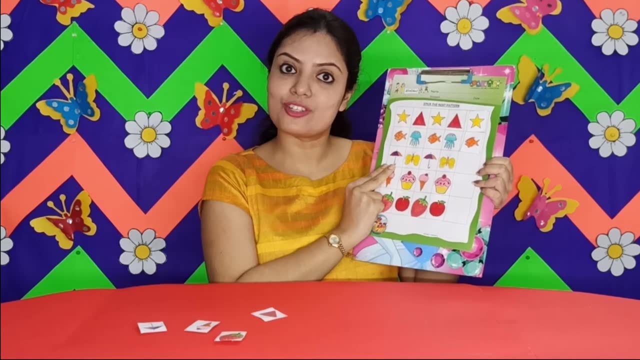 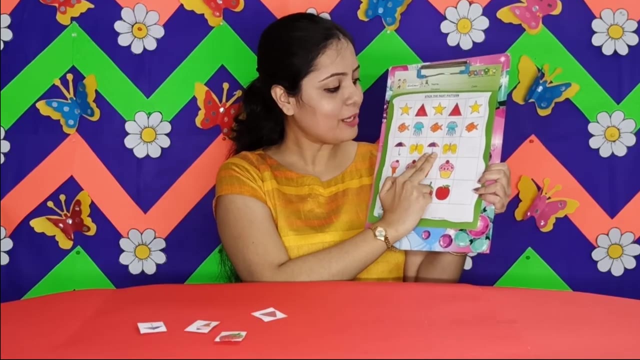 Fish, Then jellyfish, fish, then jellyfish, again fish. So our pattern is right. Okay, So the next row: There is an umbrella, followed by a butterfly. Again an umbrella, then a butterfly. So what will I put over here? 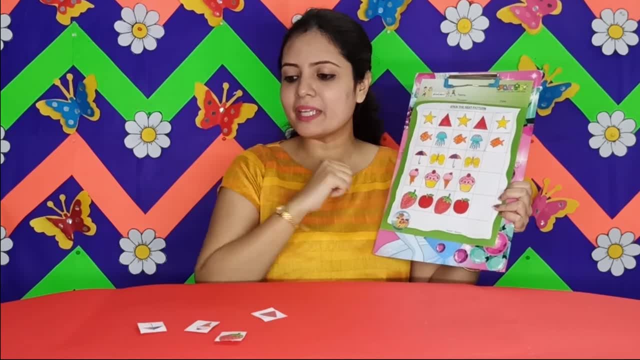 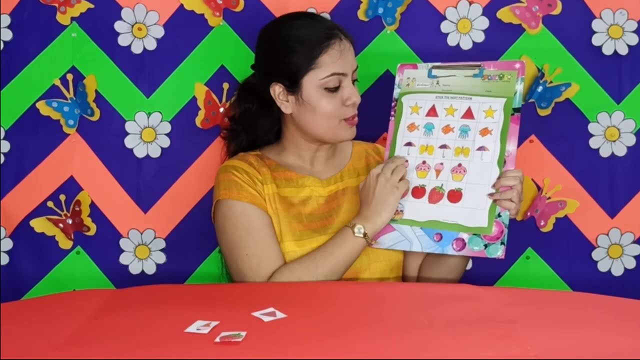 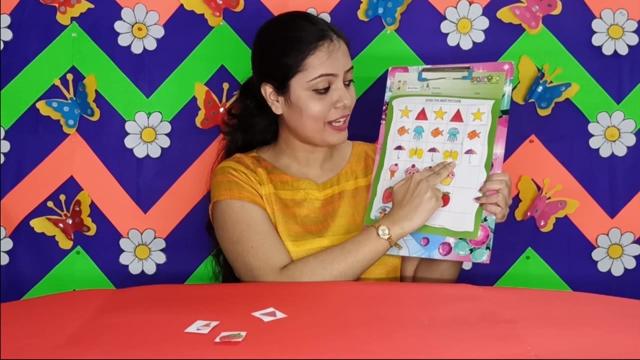 An umbrella or a butterfly. You tell me: Yes, you all are right. So I am going to place a Umbrella over here. So my pattern is complete. So umbrella, butterfly, umbrella, butterfly and then umbrella again. Okay, 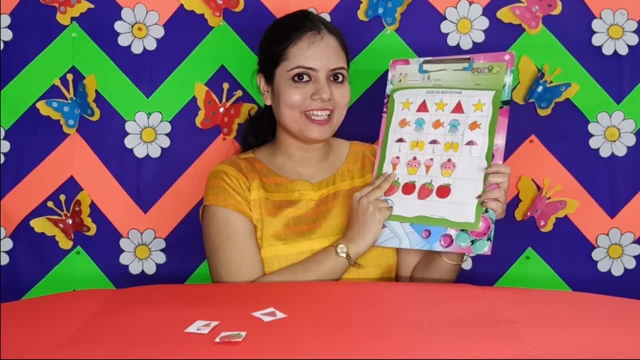 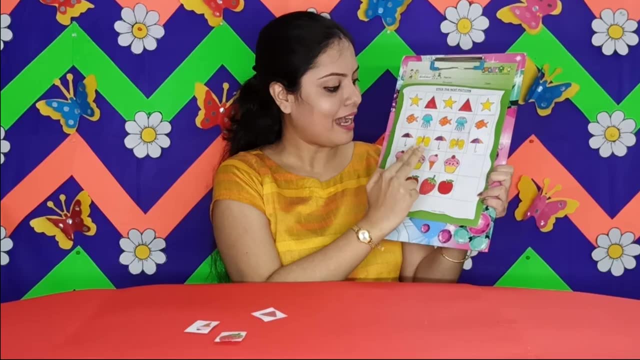 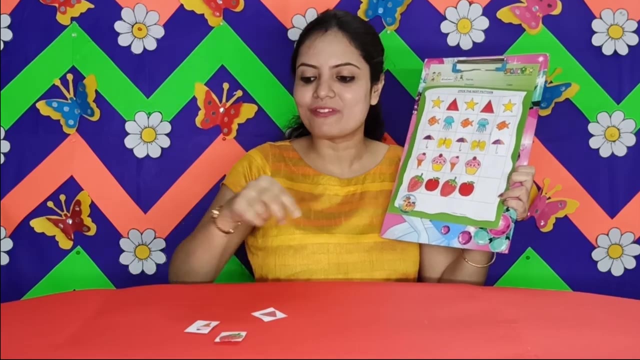 So the next one? Okay, over here we can see an ice cream, isn't it? Then a cupcake, Ice cream, cupcake. So the next one will be Ice cream. very good, So I am going to place an ice cream over here to complete the pattern. 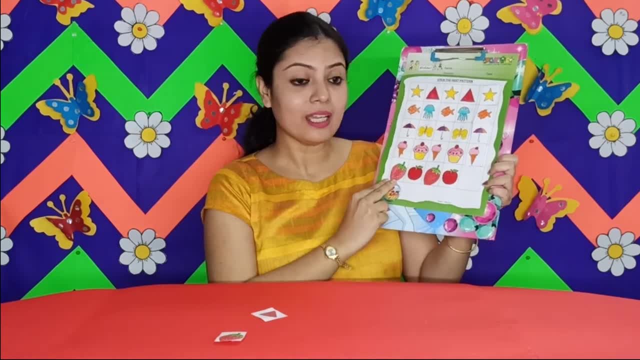 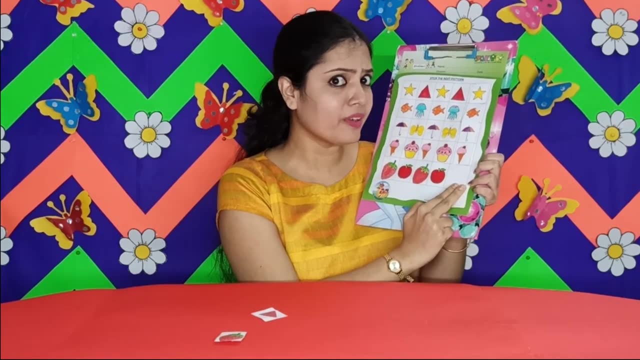 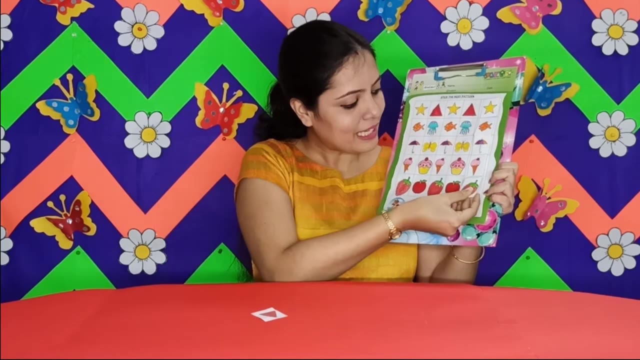 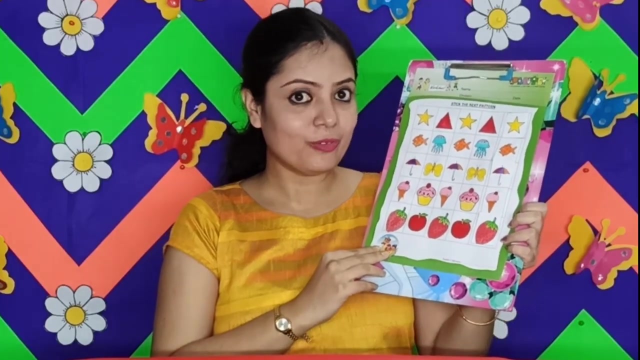 The last one. This is a strawberry and an apple. Strawberry, apple, Then apple or strawberry, Think, think. Yes, it is strawberry, So let's place strawberry over here. Okay, So our last pattern is also completed. So, children, what we have learnt today, 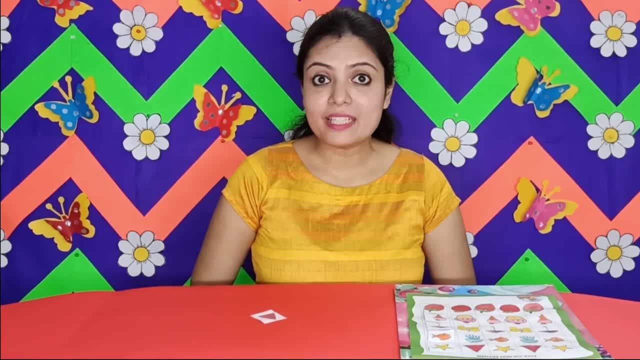 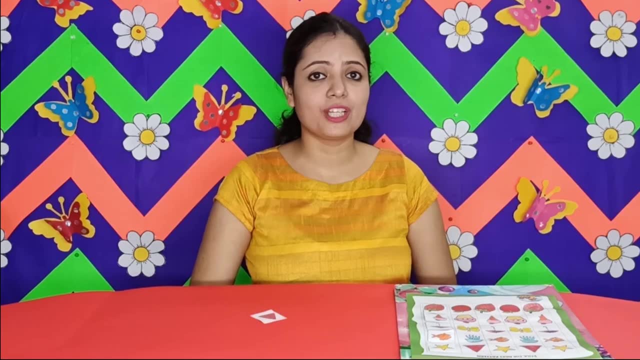 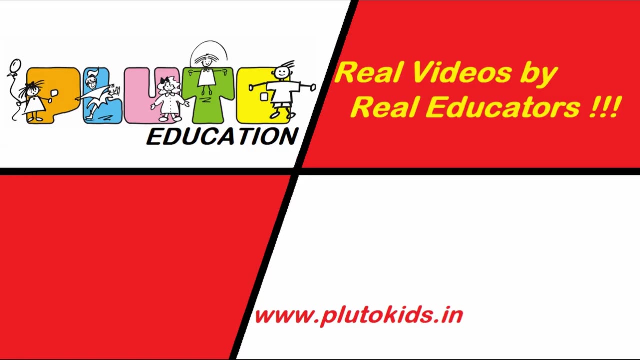 We have learnt about pattern. So, parents, this activity helps a child to develop the concept of pattern and sequence. And don't forget to order this worksheet, Thank you. I hope you love this real video by real educators. Please do subscribe to our channel.